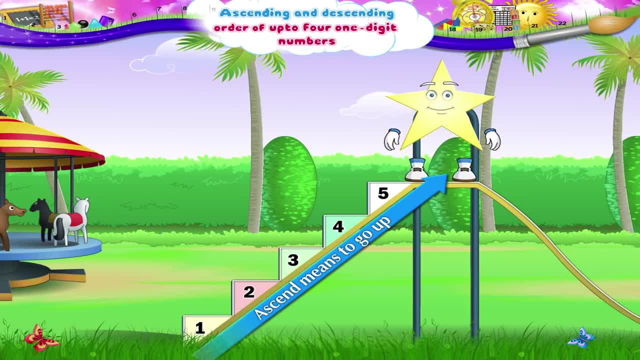 Here we are at the top Now. Starry, if you do get scared and you don't want to use the slide, you can come down the steps. Again, You can descend, But be careful: You need to come down or descend one step at a time. 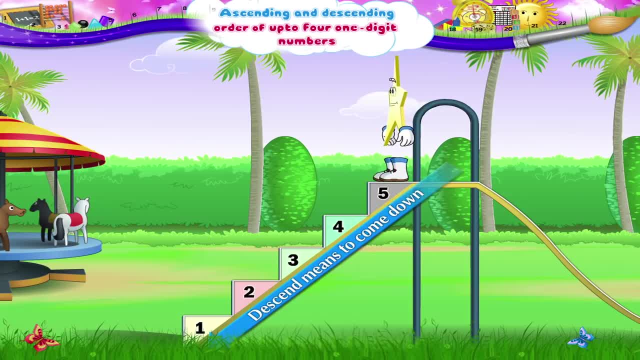 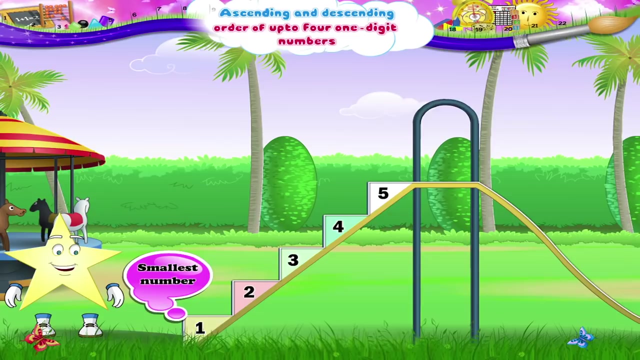 Like this: Five, four, three, two, one, And you are on the ground again. Starry, when we go from the smallest number to the biggest number, we say the numbers are arranged in the ascending order. Here one is the smallest number. 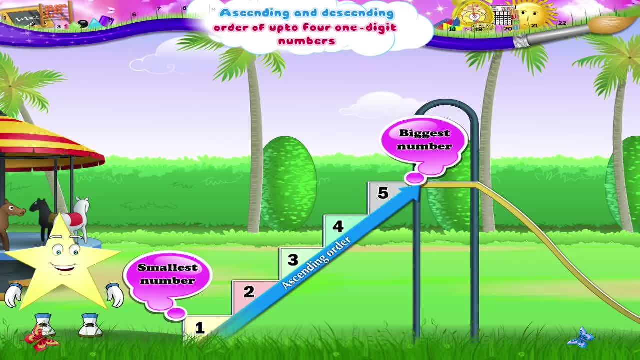 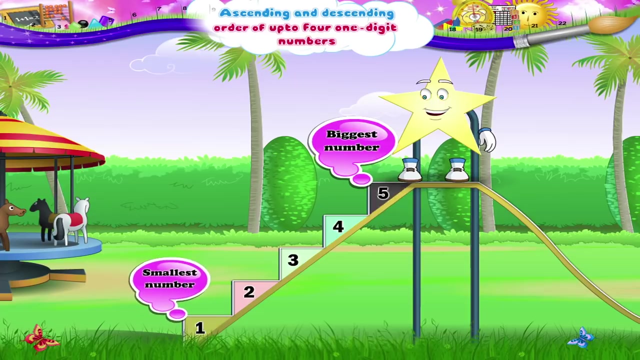 and five the biggest number And five the biggest number number. so one, two, three, four, five, ascending order up the slide and when we go from the biggest number to the smallest number, we say the numbers are arranged in descending order. five is the biggest number and one is the smallest. 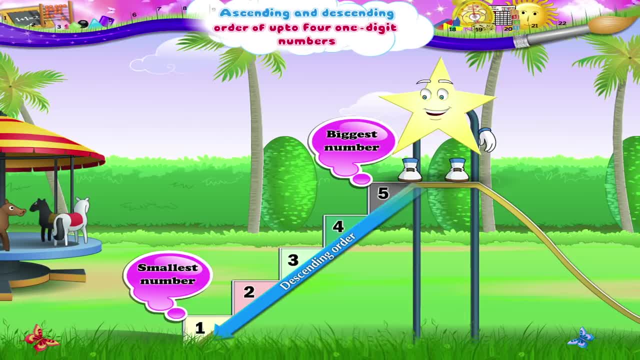 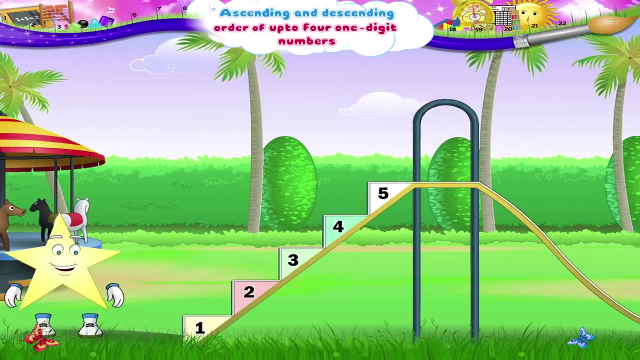 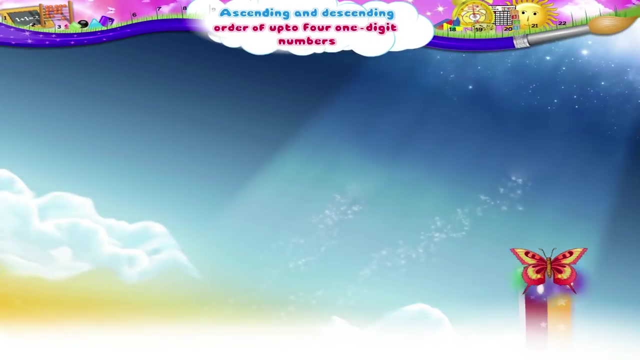 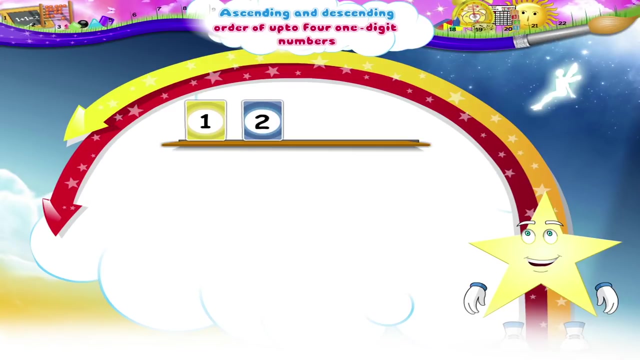 so five, four, three, two, one- descending order down the slide, starry, when you have to arrange numbers in the ascending or descending order, you first find the smallest and the biggest number. you then arrange the numbers in the middle, two, in the similar manner. take the numbers one, two, three, four. now one is the smallest number and four the 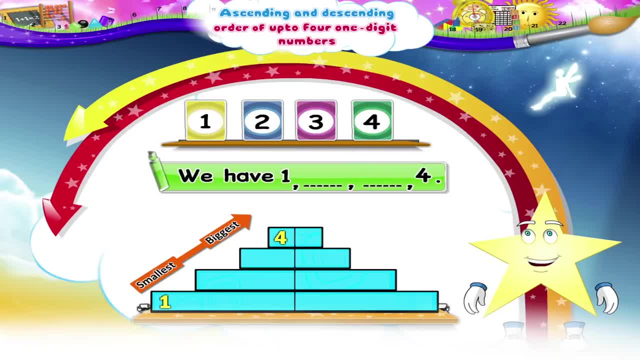 biggest. we have one dash dash four, similarly between two and four. we have one dash dash four, similarly between two and four. we have 3. 2 is the smaller number, so we write 2 in the first blank, then 3, so 1, 2, 3, 4. 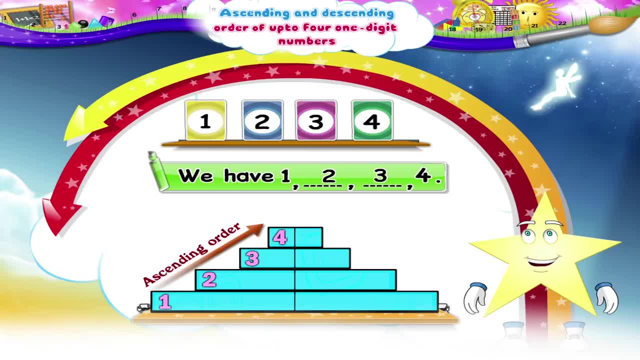 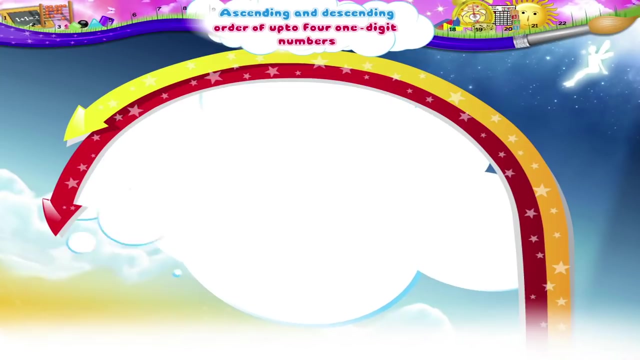 that's the arrangement in ascending order. for the descending order, we take the biggest number first and then the smallest. so 4, dash dash, 1. between 3 and 2, 3 is the bigger number. special number: we get 4, 3, 2, 1. the arrangement in descending order. 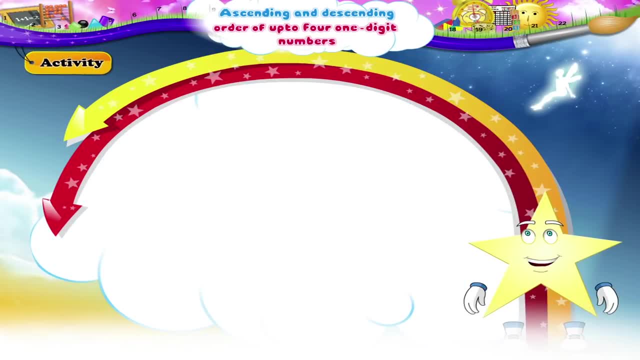 now let us do an activity together here. our sets: 1, 1, 1, 1, 2, four numbers. We have to first circle the smallest number, then the biggest number and Then put the numbers in ascending order. Shall we begin. Seven, eight, five, three. The smallest number is three. 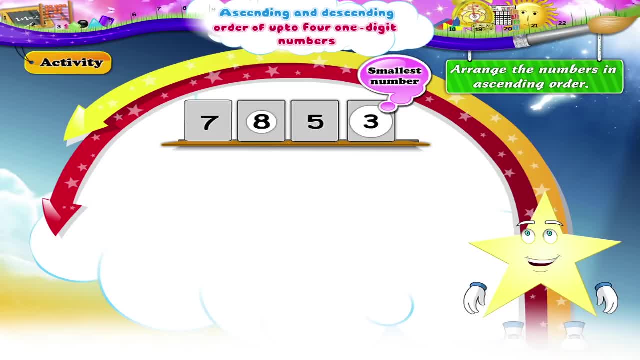 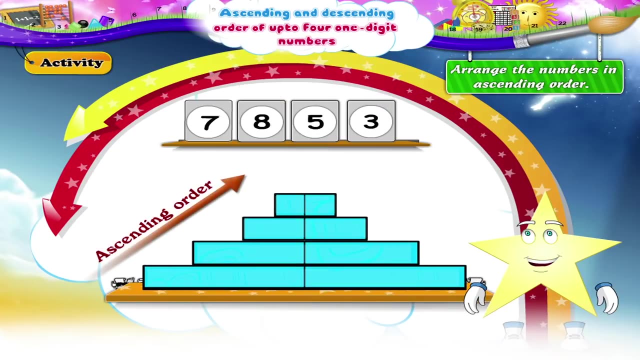 the biggest number is eight, Between seven and five. five is the smaller number. The numbers in ascending order are three, five, seven, eight, One, nine, seven, eight, four, Your starry. the smallest number is one. the biggest number is nine, Between seven and four. four is the smaller number. 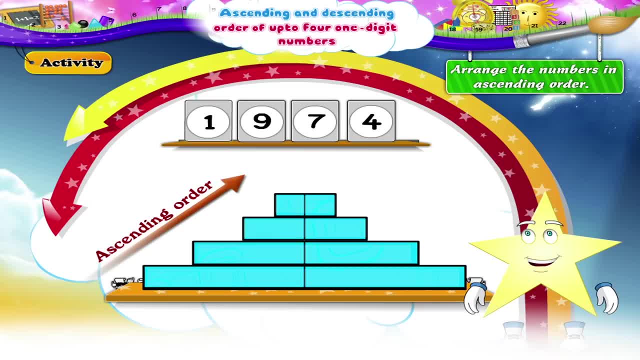 the numbers in ascending order are one, four, seven, nine, two, nine, six, five. What do you think is the smallest number, starry? Yes, the smallest number is two and the biggest number is nine. so between six and five, five is the smaller number. the numbers in ascending order are: 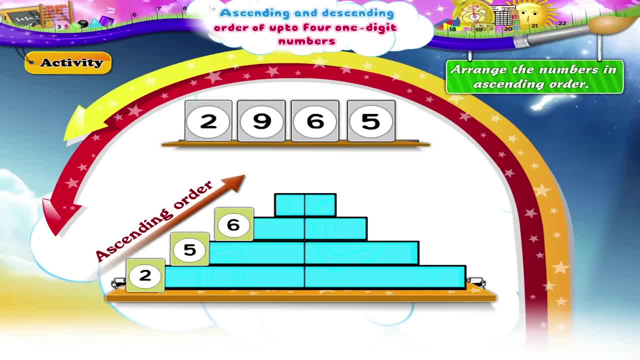 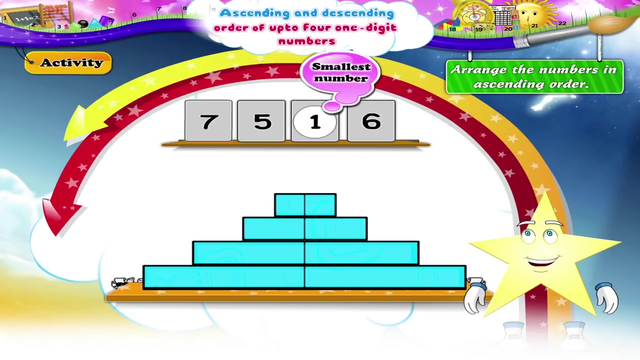 two, five, six, nine, Eight, three, four, one. here the smallest number is one and the biggest number is eight. between four and five and three. Three is the smaller number. the numbers in ascending order are one, three, four, eight, Seven, five, one, six. in this set study the smallest number is one. 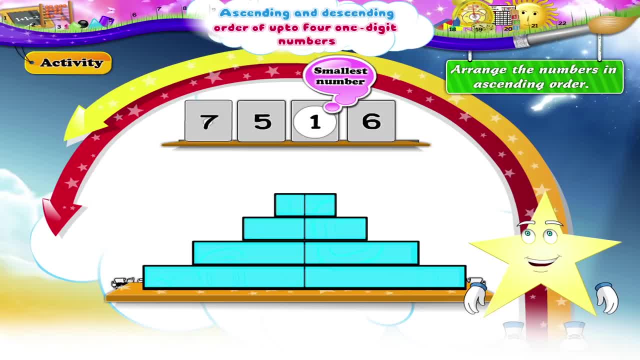 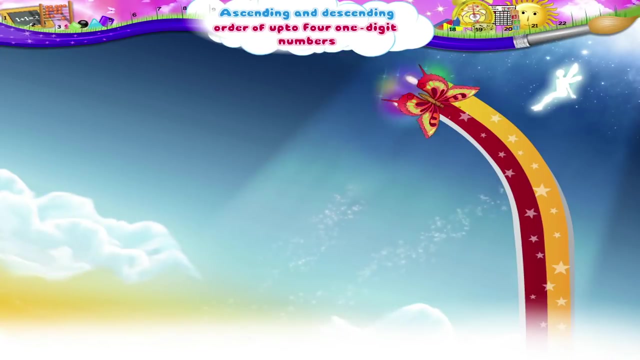 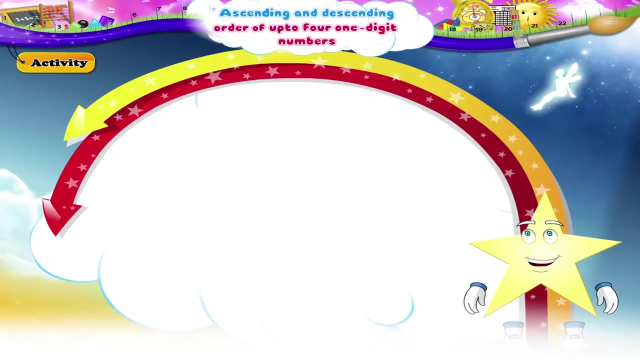 the biggest number is three, the biggest number is seven and between five and six, five is the smaller number. the numbers in ascending order are one, five, six, seven, and in this activity study, we have to first circle the biggest number, then the smallest and then put the numbers in descending order. let's begin seven, nine. 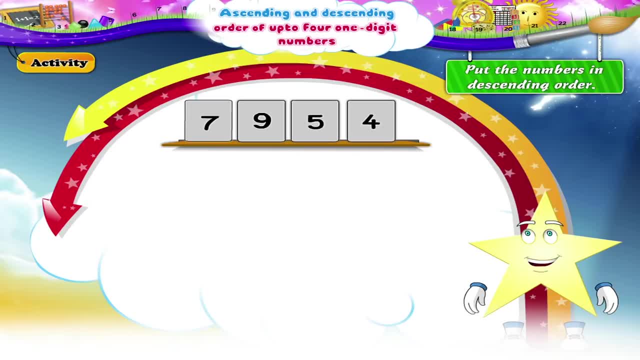 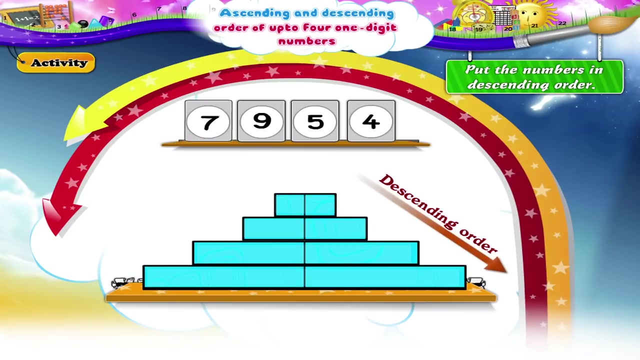 five, four, seven, nine, five, four, starry. the biggest number here is nine and the smallest number is four. between seven and five, seven is the bigger number. the numbers arranged in descending order are nine, seven, five, four, 2,, 3,, 5,, 9. 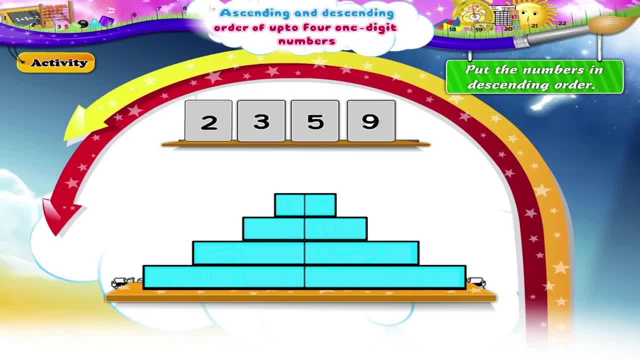 The biggest number is 9.. The smallest number is 2.. Between 3 and 5,, 5 is the bigger number. The numbers arranged in descending order are 9,, 5,, 3, 2. The next set of numbers is: 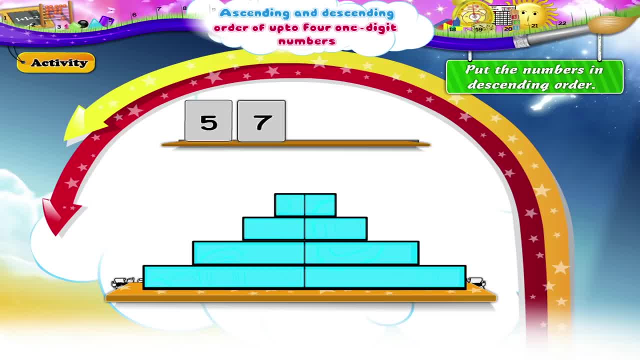 5, 7,, 1, 8. The biggest number is 8.. The smallest number is 1.. Between 5 and 7,, 7 is the bigger number. Study: The numbers arranged in descending order are 8, 7,, 5, 1. 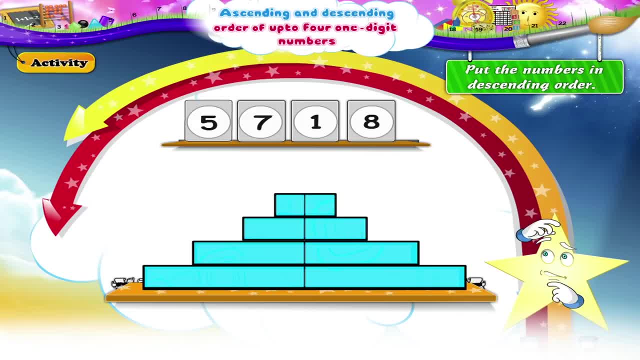 Study: What about 6, 8,, 3, 2?? Yes, the biggest number is 8. And The smallest number is 2.. Between 6 and 3,, 6 is the bigger number. The numbers arranged in descending order are: 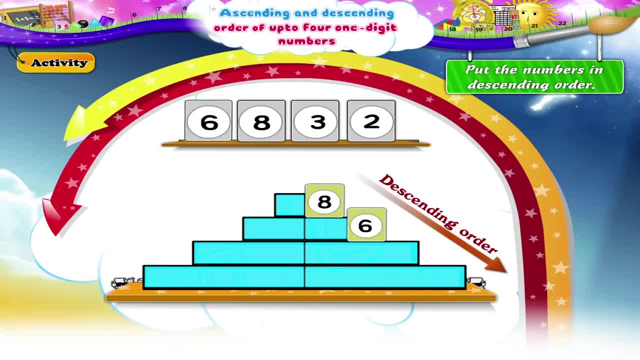 8,, 6,, 3, 2. Finally, the numbers 1,, 6,, 7,, 2, 8,, 6,, 3,, 2: The biggest number is 7.. The smallest number is 1..